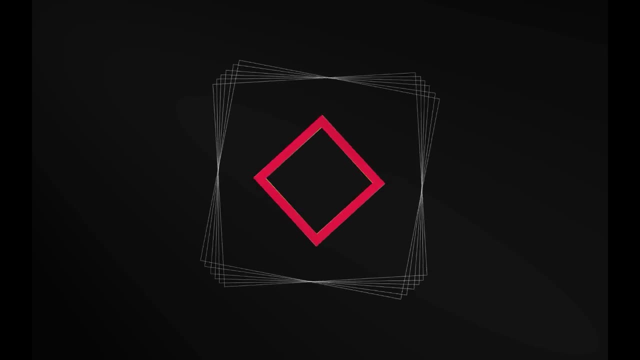 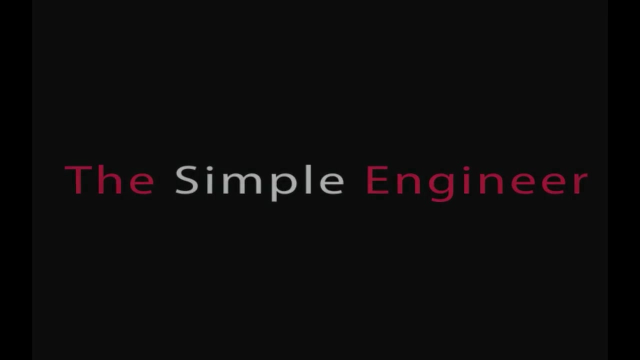 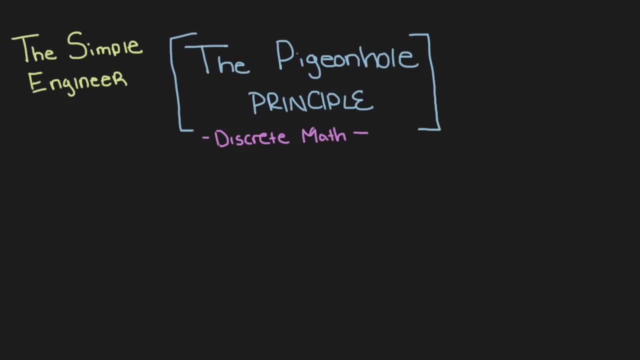 What is going on, guys? Welcome to another video brought to you by The Simple Engineer. Today we are going to delve into the topic of the pigeonhole principle, which is very common among discrete mathematics, especially with computer science relevant topics. So let's go ahead and get started. For those of you who don't know, this is really a powerful 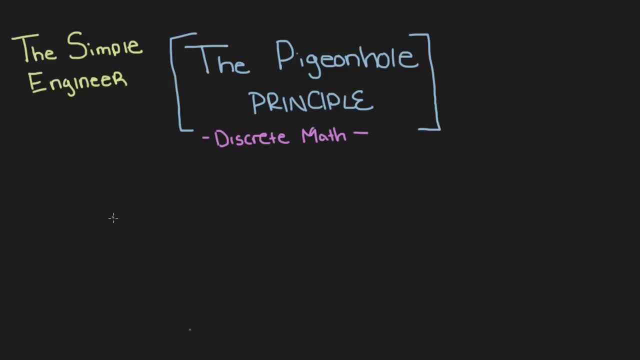 tool in combinatorial mathematics And it basically states that if you have three pigeons and available are two different boxes, then is it possible to put all three pigeons in these two boxes? And the answer is yes, but there's a slight condition, and that's that. 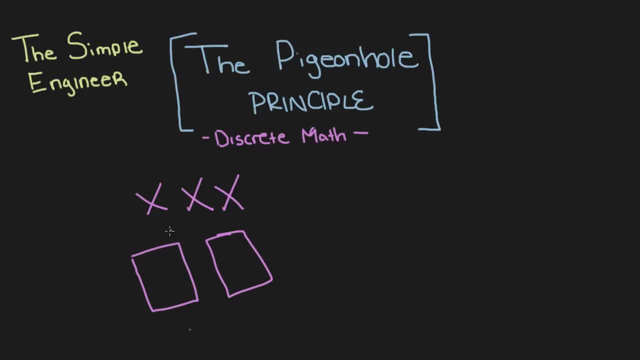 one box must contain at least two pigeons. So I put one pigeon here, but this box has to contain these two pigeons. Okay, So it's a very, very trivial idea, It's not, it's not hard to understand. but 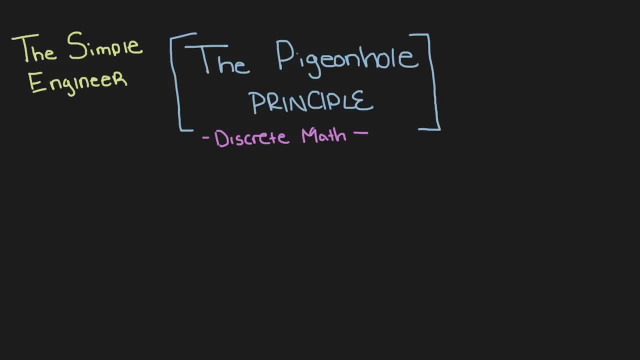 there's different ideas underlying this um topic that make it a little more non-trivial. So another kind of kind of basic example is among three people. So let's say we have three people at a party. Okay, There's only two types of genders, male and female. So we're 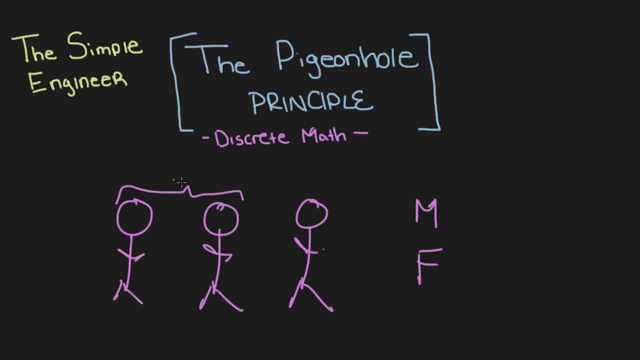 saying that That at least two of these people must be the same gender. Okay, So another very, very simple idea: because you can't have three people all being different genders, because there's only two possible genders, Okay. So now let's kind of delve into how to solve these types. 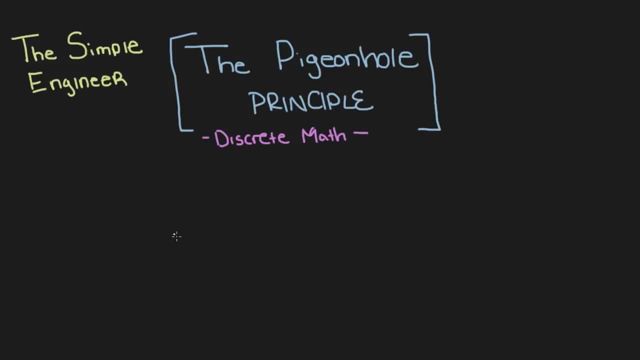 of problems. What kind of formulas are presented to us under certain circumstances? Okay, So it really says that if in pigeons are an M Boxes, Okay So you have in pigeons, in pigeons, in M boxes, such that in is greater than M. 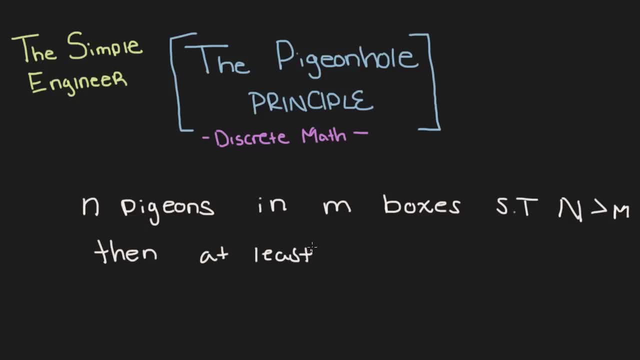 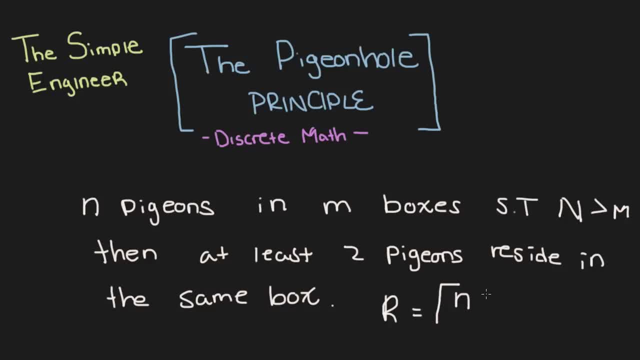 the ceiling function of in pigeons over M Boxes. Okay, So the ceiling function basically states that if I have any numbers, say 2.0001, one or 3.5, the ceiling of 3.5 would round to four and the ceiling of 2.0001 would round to. 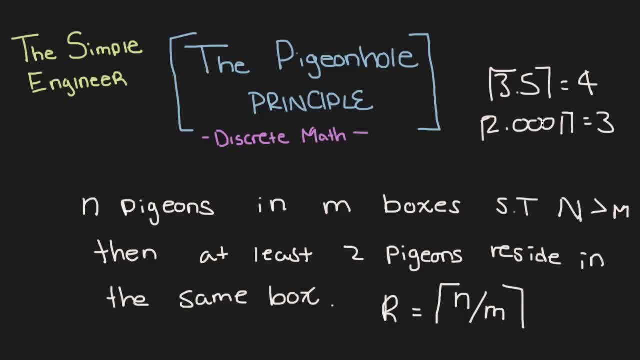 three, et cetera, et cetera. You get the idea that it rounds up: Okay, From whatever the numbers. However, if I just had the ceiling of two, this equals two, because there is no number that's even slightly higher than two, So it just stays at itself. Okay, So that's what the ceiling says. 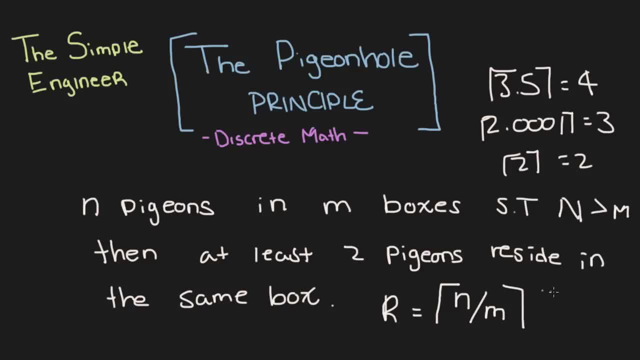 So if I have the ceiling of three pigeons but I only have two boxes, well, what's the ceiling of three over two? This is 1.5, and the ceiling of 1.5 equals two. So it's saying that I have to have. 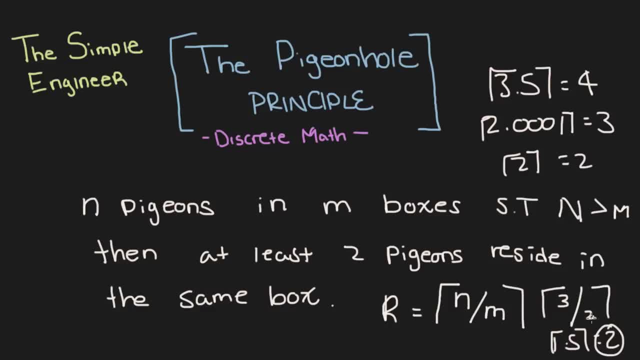 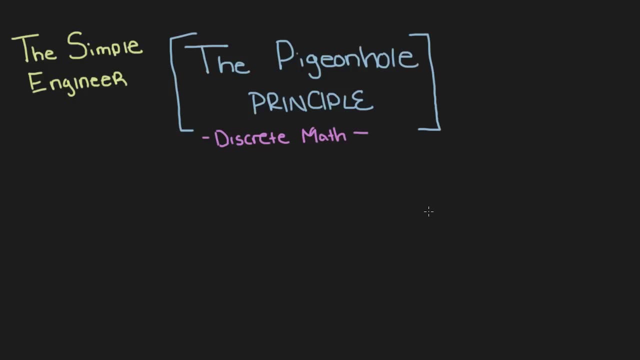 at least two boxes, Okay, Present for this to hold true. Okay, So now let's get into some actual examples. So I'll go ahead and erase this definition And we will once again place these equations. So I initially said that r equals the ceiling of n over k. Okay, Where? well recently, well previously. 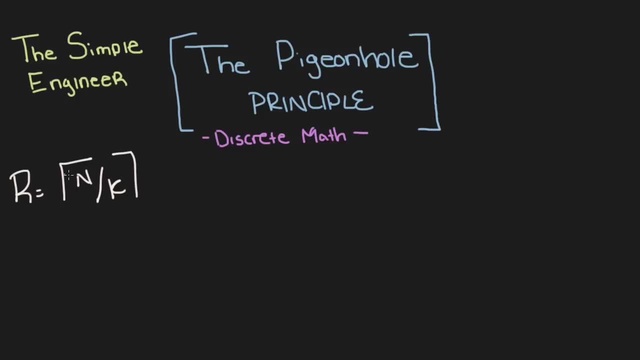 we used m, okay, m boxes, But now we're going to use just a generalized formula So we can keep this uniform. Okay, so we're going to keep this universal here. So our I like to think of as the, whatever, the. 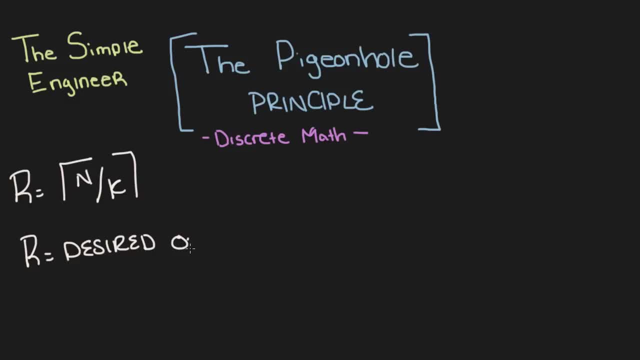 desired output is. So this is going to be our desired output, if you will. And then n equals the number of items, number of items, and we're going to say the number of items is, metaphorically, these pigeons, and we'll say k equals the number of. 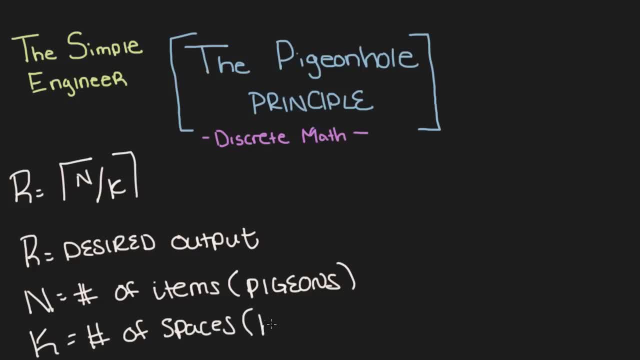 spaces, which would technically be the boxes, are the pigeon holes that these things can be placed in. And keep in mind that this formula here is the same mathematically represented as n equals r minus one times k plus one. these things mean the same thing. So when you have certain variables, 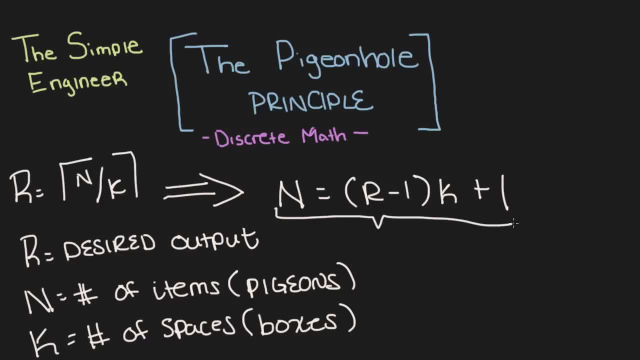 that are unknown or hard to find, then you can use this characteristical equation, character equation, and it'll give you certain variables that you could not otherwise find using this. okay, so keep these in mind. you have equation number one here and equation number two here. 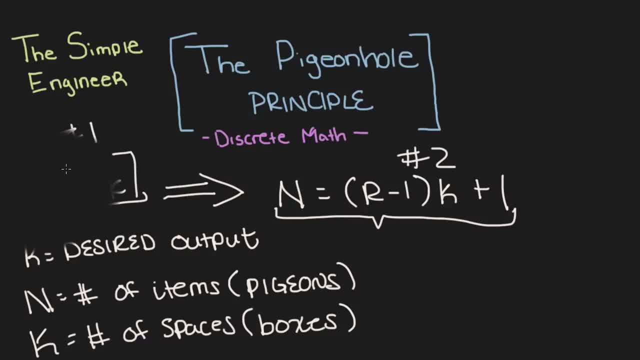 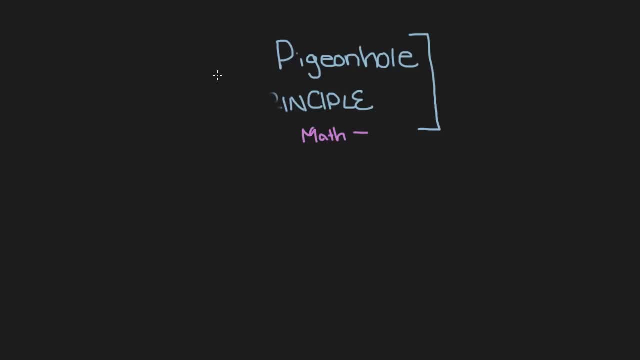 and you'll probably want to write these down for some of the examples that we are going to do in this video. okay, i'll actually go and erase all of this, so let's do a couple examples. we'll start with a more trivial idea. so say, we have for every, for every, 27 word sequence in a book. 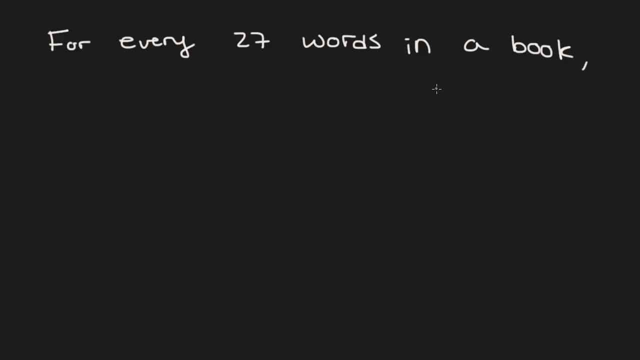 27 words in a book, at least two words begin with the same letter. at least two words begin with the same letter. okay, we want to prove that this is true. okay, so, um, we'll kind of revert back to our idea that, um, the number of pigeons. 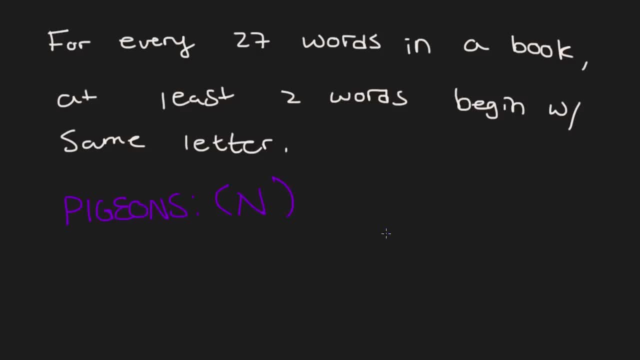 which is represented by our in value, the number of pigeons, is equal to the 27 words. and then if the number of boxes or rows, and also, if we're using the same metaphor, the number of boxes we have, which we denoted by k, is equal to the 26 letter combinations that we can have from the 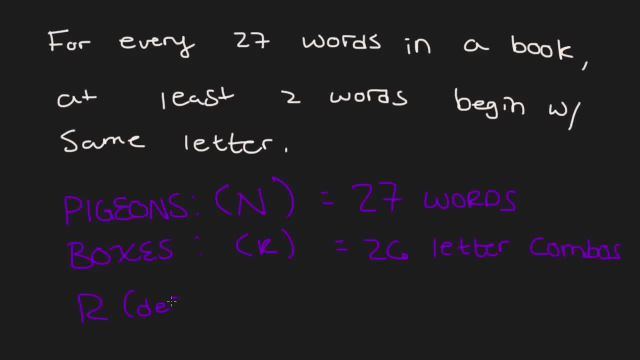 letters in the alphabet. so our desired output- i like to think of r as, whatever our desired output, the ceiling of n over k, which is equal to the ceiling of 27 over 2, which indeed equals 2.. So we proved that at least two words begin with the same letter By solving this equation. 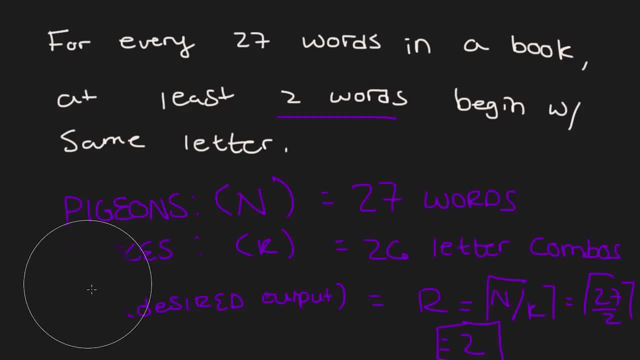 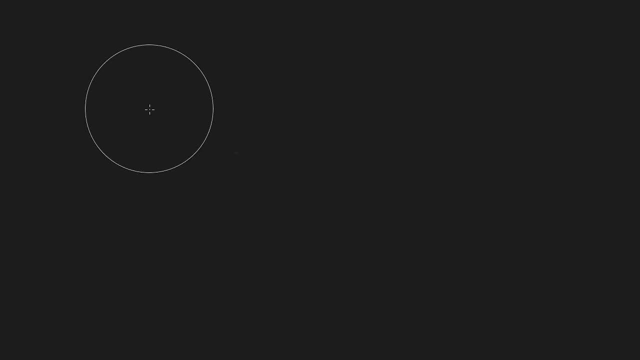 you see, 2 equals 2, and therefore the proof is satisfied. Okay, so that was a more. that was a trivial example, not too hard to understand, basic proof. So now we'll look at something that's a little harder to grasp, and this is our bowl example. So we have a bowl. 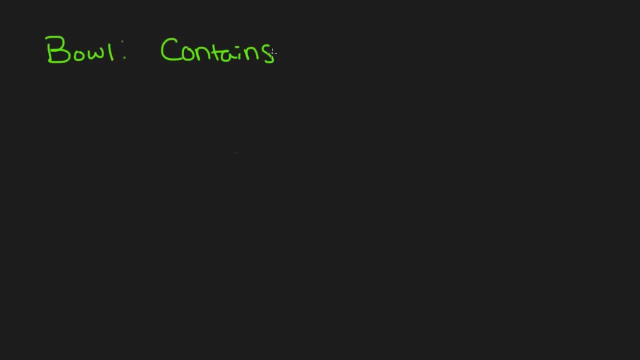 and this bowl contains six red balls and it contains six blue balls. Okay, and a woman is selecting these balls blindfolded. She's selecting these balls blindfolded and we want to know what is the minimum. what is the minimum balls to select? 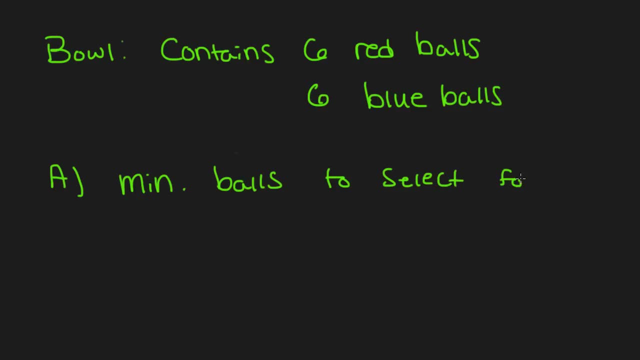 for at least three blue balls. at least three balls. Okay, so you want at least three blue balls, and something to consider in the pigeonhole principle is: you always want to consider the worst case scenario. So if the minimum balls to select for at least three balls, 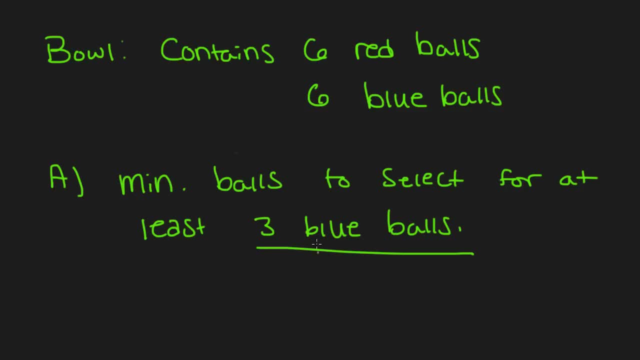 to for sure have, for sure have. then we need to select nine balls, and that's because, worst case scenario, we could select all six red balls, which would put us at count six. However, we want three balls that are blue. So once we exceed the six count, then all we have left to select are the 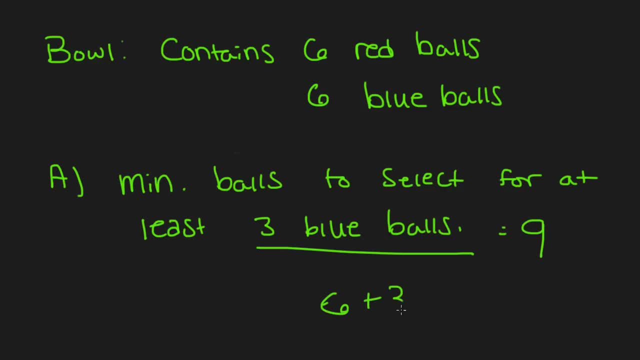 blue balls, and we want three of them, So we would just do six plus three, and that's how we get nine. Okay, so once again not too bad. but now let's go ahead and do something a little trickier. 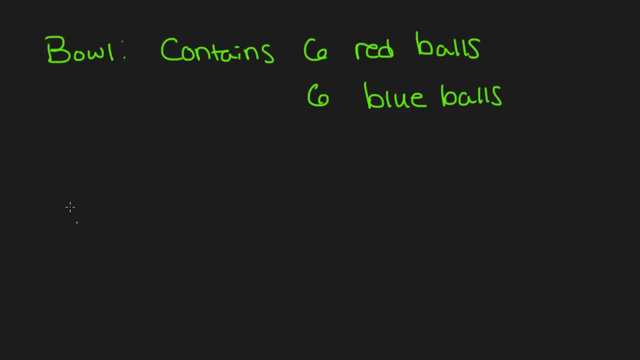 So we have the same set here, but B is saying the men to have three of the same color. Okay, so this is a little different because you could have either three of the red or three of the blue. So we can actually go back to our equation to help us solve this. And we said that our 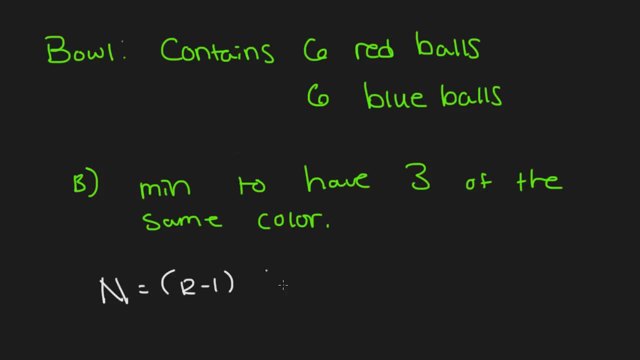 equation was: n equals r minus one, multiplied by k plus one. Okay, so, like I said, I like to think of r as the desired output, k as the number of boxes and n as the possible, like the pigeons in the situation. 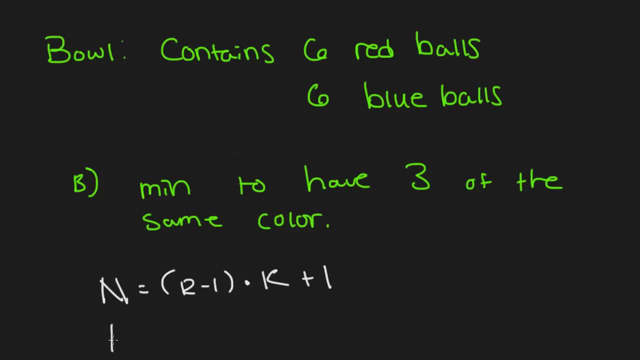 So the minimum number, which would be technically the pigeon's n equals r, so the desired output, which is given to us as three, so we could go three minus one times, and then the number of boxes that we have, which is two, because we have two different types of colors. 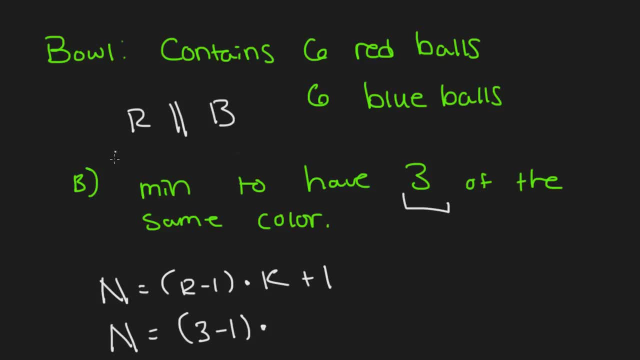 We can either have red or blue, which would be the two different types of boxes, if you will. So we have two different types of colors or categories plus one, And this is equal to two times two, which is four plus one equals five. 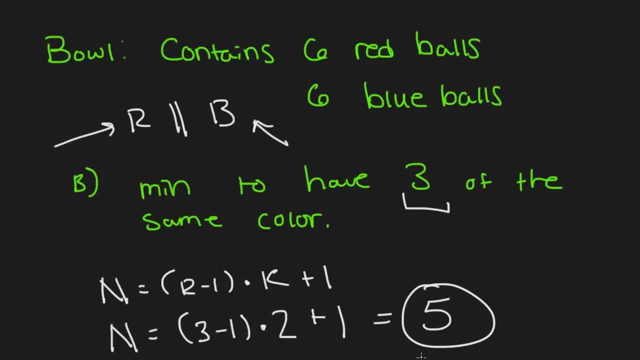 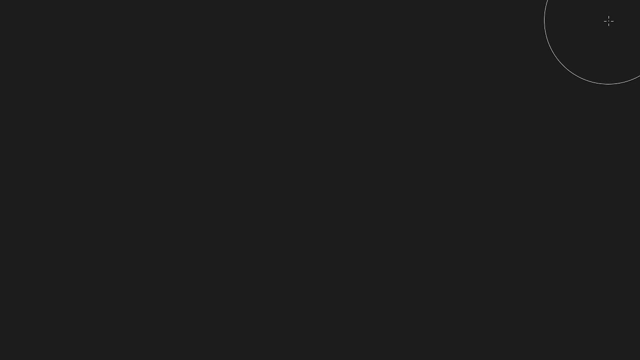 Okay, So we have five different draws that we have to do to ensure three of the same color. Okay, So quickly moving along so we can get through all of these examples, we are going to go ahead and do something that we call bit strings. 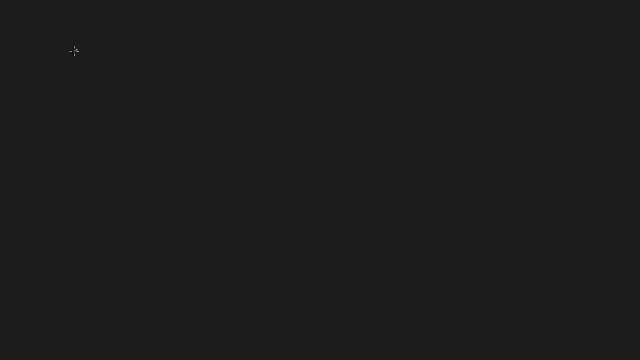 Or utilize the idea of bit strings. So we have four different types of bit strings And, for those of you who don't know what a bit is, it's basically a sequence of numbers that are either zero or one. Okay, So we have a bit string of zero. 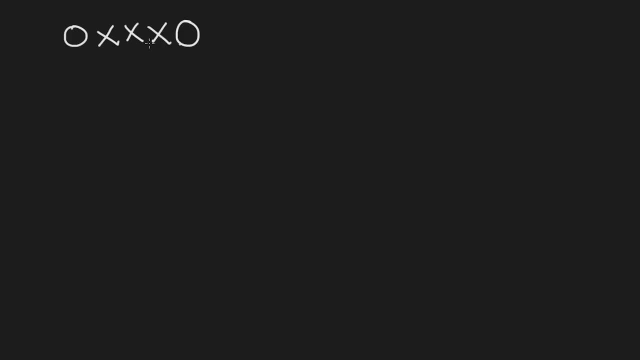 and it follows this structure. Okay, so we can have two zeros on the end and we don't care if zeros or ones are in the middle. We can have a zero in the beginning, don't care what's in the middle, but we have a one at the end. 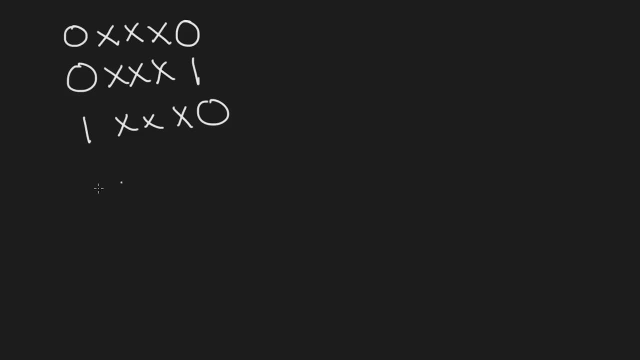 We can have a one at the beginning, don't care what's in the middle, and a zero at the end. Or we can have a one in the beginning, don't care what's in the middle, and a one at the end. 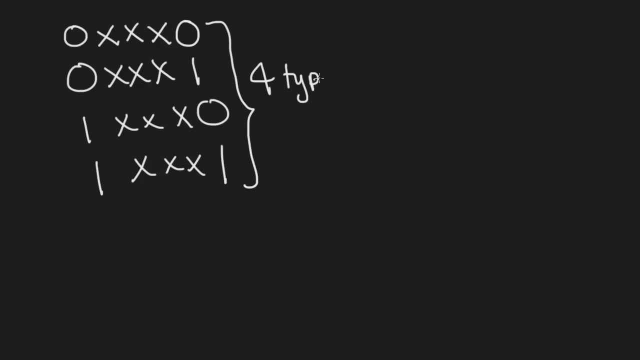 So we have these four different types of structures- okay, Four types, And they consist of five different numbers, And they wanna know how many bit strings, how many bit strings, we need to select five of the same type. Okay, so we want five of the same type. 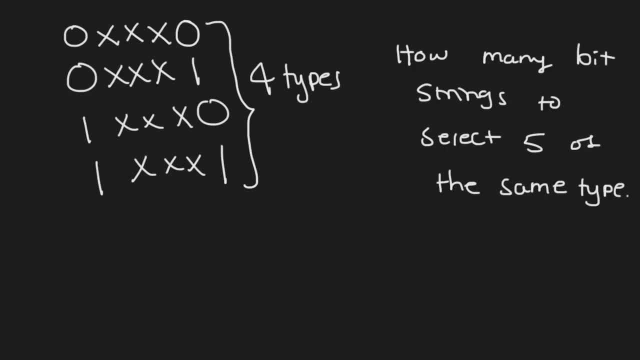 So keep in mind- I always like to refer back to this equation- how I think of these types of problems. So we want five of the same type, which would be our desired output. So in the equation we would say: r equals five. 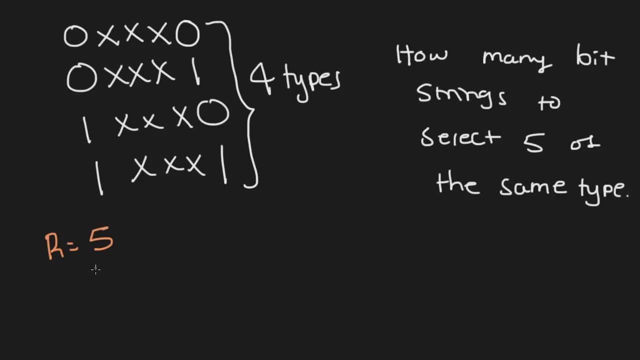 because that's the desired output, And then the different types of boxes or possible places that we can put. this is four, okay, Because we have four different types. So we can have four different types of these bit strings. So k is equal to four. 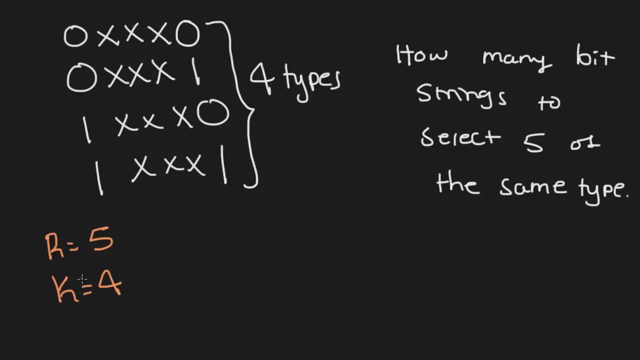 Now we don't know the number of pigeons or the amount of bit strings to select five of the same type. So that would be n equals and then our unknown. So we could follow the formula n equals r minus one times k plus one, and then we would just plug this in: r equals five minus one times four plus one. 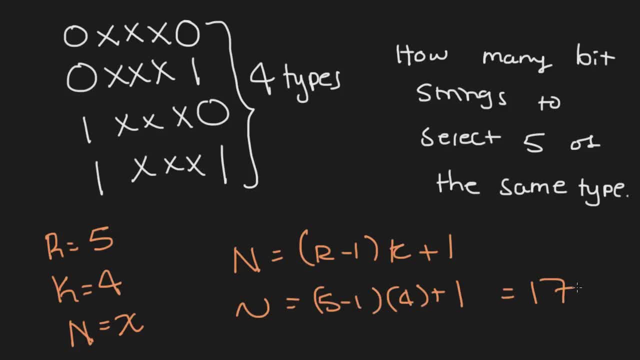 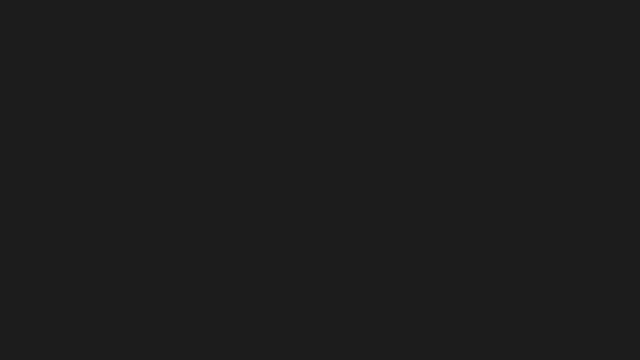 And that would equal 17. Okay, so 17 is the number of bit strings to select to have five of the same type. Okay, now let's move on to our next example. Okay, so our next example says that we want five of the same type. 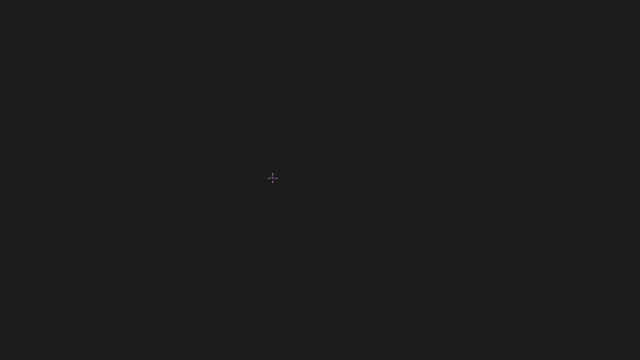 Okay. so our next example says that we want five of the same type. It says that we can have three. Okay, so we have three letter words printed and they cannot repeat. So a computer is printing out these three letter words and none of these letters can repeat. 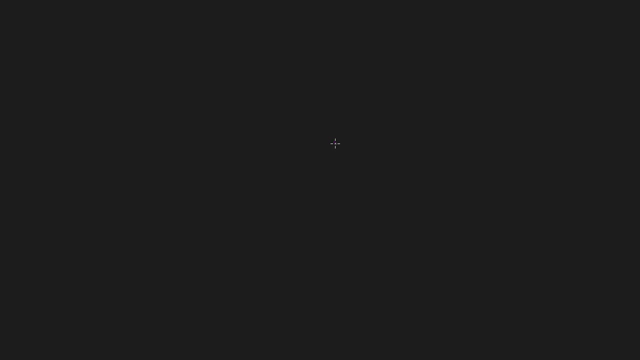 And it wants to know how many words to print to ensure that eight of these words that are being printed out are identical. Okay, so we have three letter words and they can't repeat, So we're going to actually figure out how many three-letter words there exist that cannot repeat. 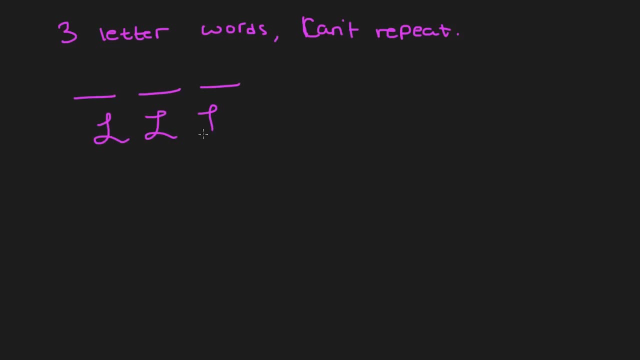 We would just say: okay, we have three spaces, they're all letters and they can't repeat. So the first letter could be any of the 26 letters in the alphabet. Then the second letter would have to be 25 letters because it can't intersect with the first letter. 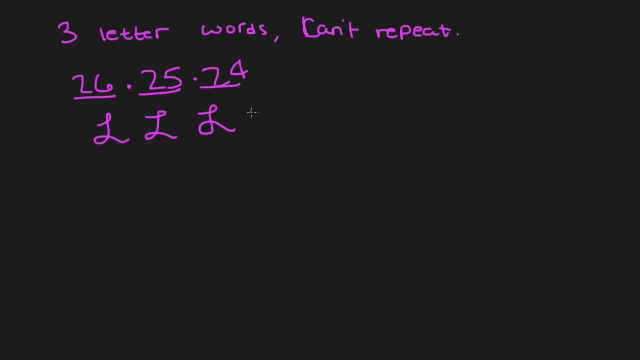 And then 24 letters for the third one, And we would just multiply these out. And if we multiply these out we would get 26 times 25 times 24, which equals 15,600 possible combinations for three-letter words that cannot repeat in the English alphabet.